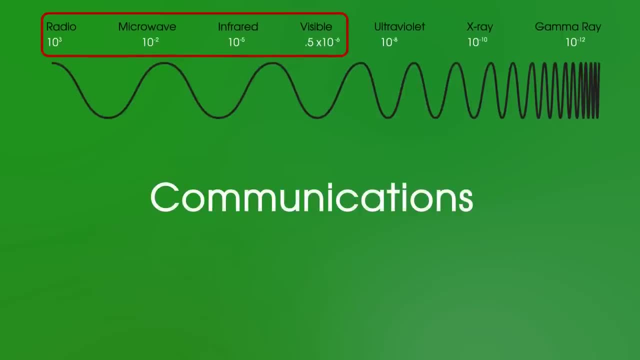 All these parts of the spectrum are used to generate light. Radio waves are used in communications. Radio waves are used for sending TV and radio signals, both short and long distances. Really, short wavelengths are used for very short distances and the longer wavelength for longer distances, as they can reflect off a layer of charged particles in the atmosphere called the ionosphere. 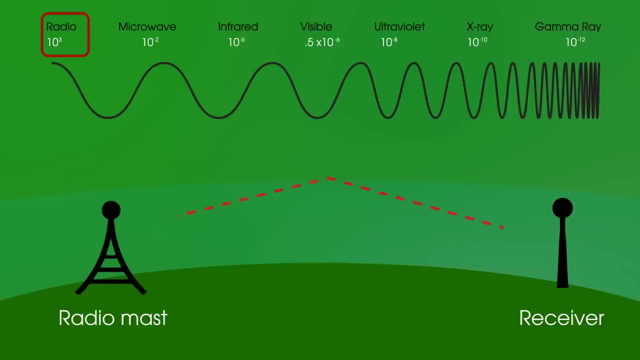 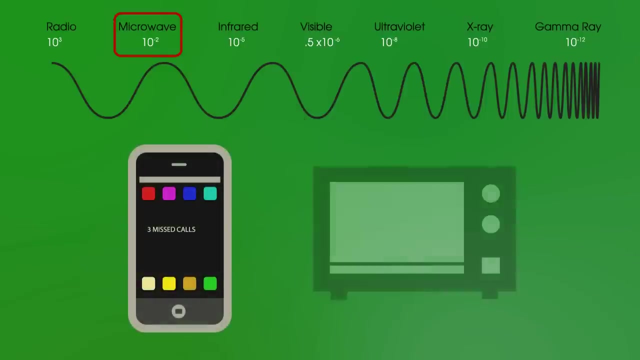 However, radio waves can't pass through the ionosphere, so if we want to communicate with satellites, we must use microwaves, as they will easily pass through the ionosphere. Microwaves are also used in mobile phones, and certain wavelengths are absorbed strongly by water molecules and so are used to cook food. 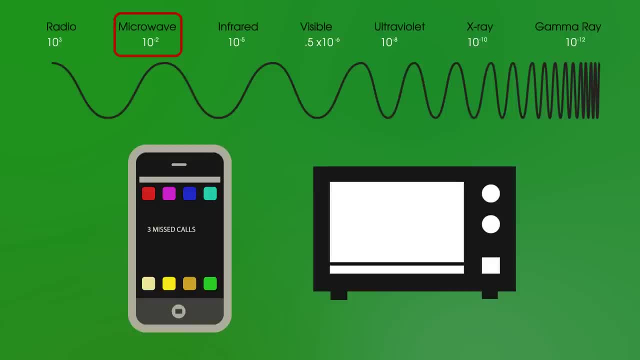 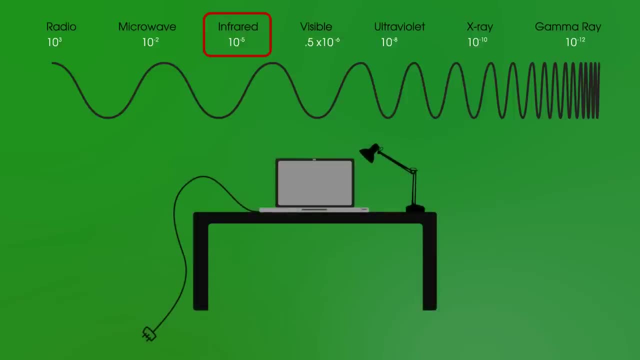 These are not the wavelengths, however, that are used in mobile phones. Infrared, as we know, carries heat and can be used in thermal imaging and for grills for cooking, and it is also used in communications. as is visible light. 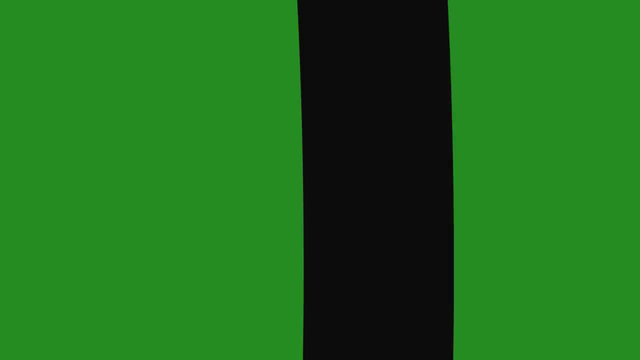 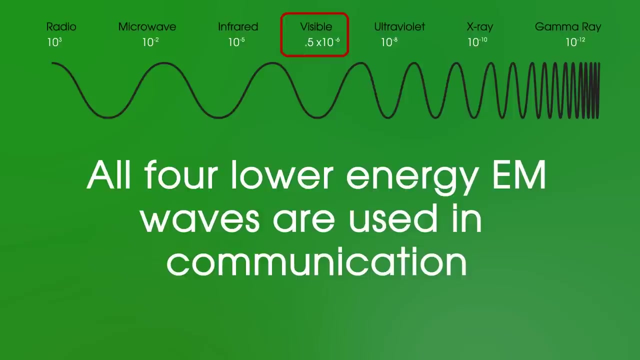 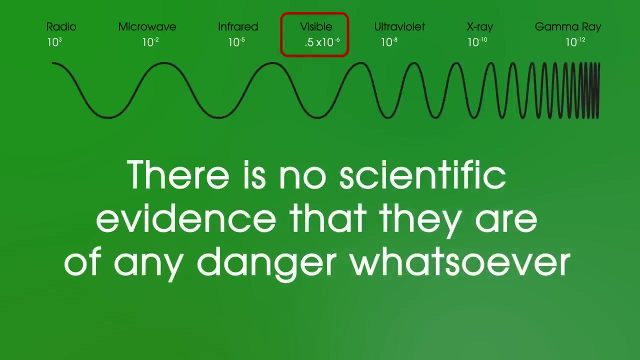 Both are being sent down optical fibers. So all these four lower energy electromagnetic waves are used in communication. but is there any danger in using them? Well, at the moment there is no scientific evidence that any of these parts of the EM spectrum pose any danger whatsoever, apart from maybe getting burnt by infrared. 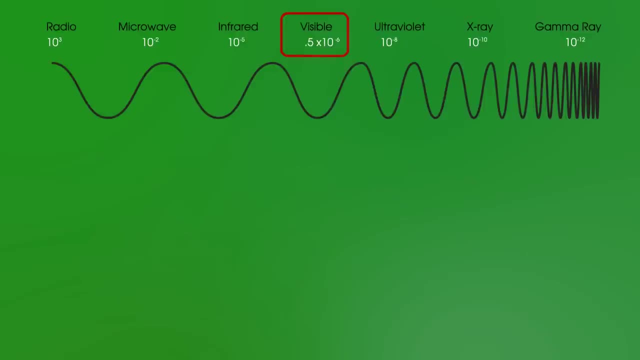 Now let's move on to look at the high energy part of EM. So what are these used for? Well, ultraviolet is used in sunbeds to help you get a suntan, and it's also used in special security inks, because they absorb ultraviolet and emit visible light. 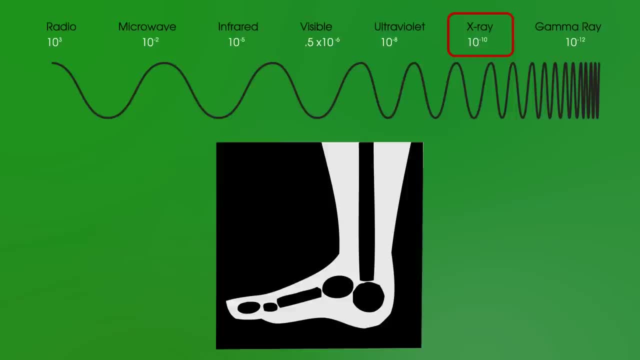 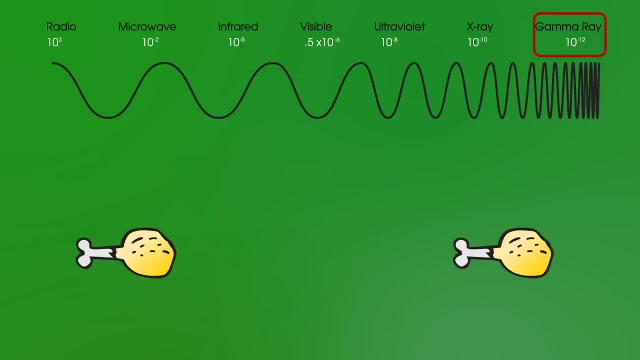 X-rays, obviously, are used to look for broken bones in hospitals. And finally, gamma rays are used to kill bacteria in food, to keep it fresh longer, to sterilize surgical equipment and also to kill cancer cells in radiotherapy. Now, this is the high energy part of the spectrum, so there are dangers with using these. 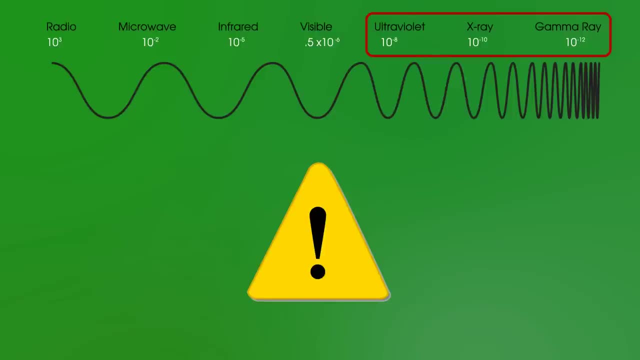 As you know, too much exposure to ultraviolet can cause skin cancer. Now X-rays and gamma rays are even more dangerous, as they have enough energy to remove an electron from an atom, creating an ion. We call this ionization, And this can really damage cells and can actually kill them.